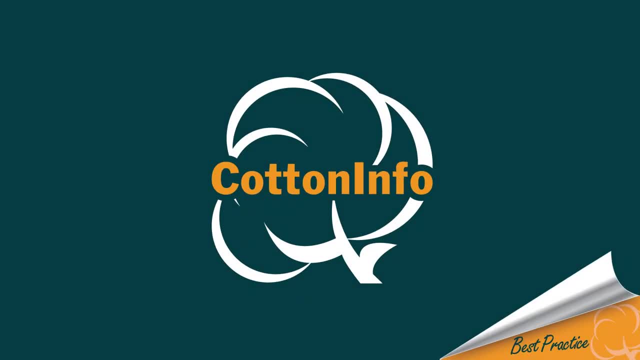 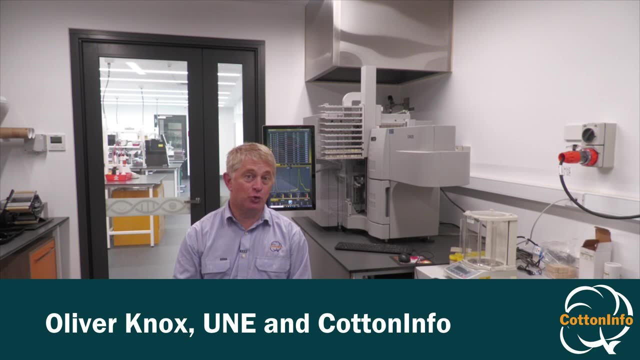 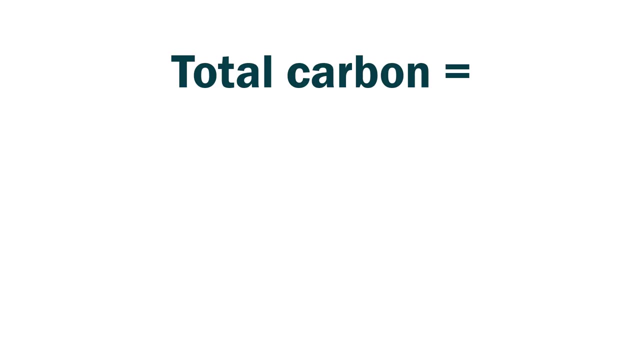 Hi there, Some of you have been asking questions about carbon, So we wanted to give you a brief video to basically talk through some of these things about carbon. One of your first questions is: what is total carbon? Well, total carbon is the organic carbon and the inorganic carbon. that 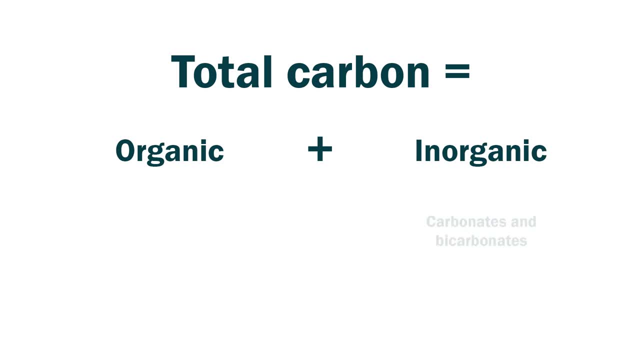 we find in our soils. The inorganic carbon is basically the carbonates, And when we look at a soil and it maybe has high carbonates, we try to remove those using acids, Because what we're interested in is the organic stuff. Now this exists as our soil organic matter And what that. 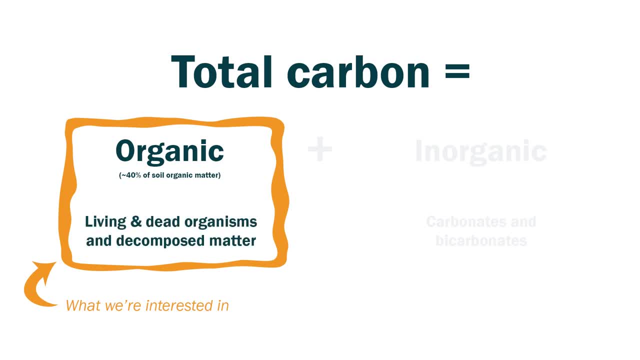 is is basically the form of plants, bits of animals, all that dead stuff that's turning over in our soils and also the life that's in our soils at the moment. But it's really hard to measure soil organic matter. So what we generally do is we measure soil organic carbon. Now 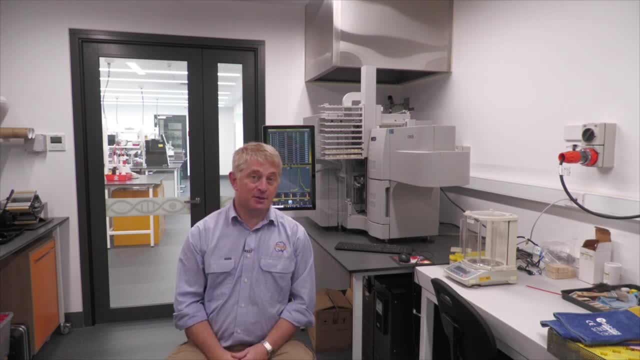 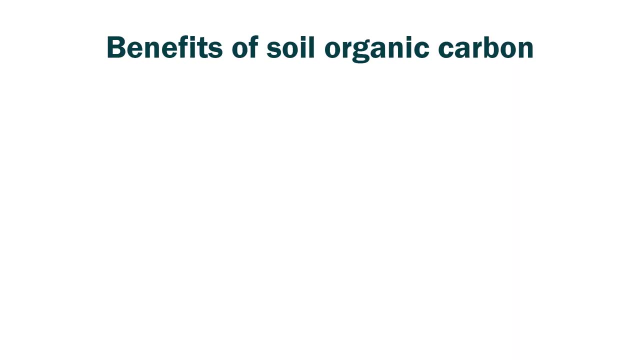 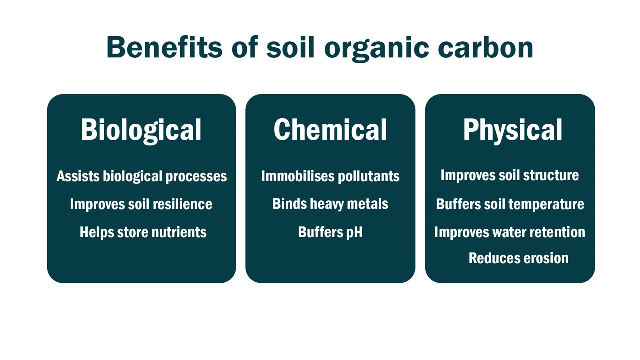 soil organic carbon is only about 40% of the soil organic matter, So we use an estimation or an approximation of our soil organic matter based on those organic carbon measurements. Soil organic carbon is important because it's the food that basically feeds the biology that drives the nutrient cycles which we rely on to grow. 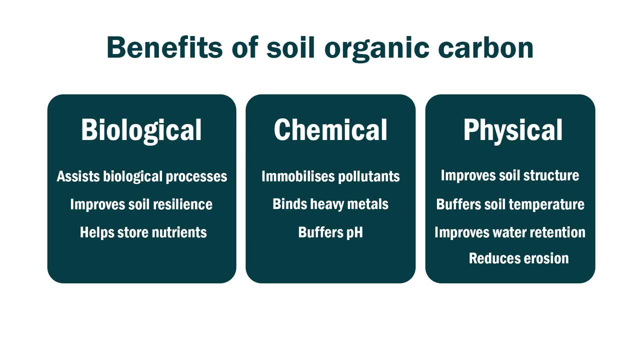 our plants. It also acts as a type of glue, helping to stick the mineral component of our soils together, And in doing so it gives us structure. And that structure allows better aeration and also can help mitigate some of the effects of erosion events. And I guess 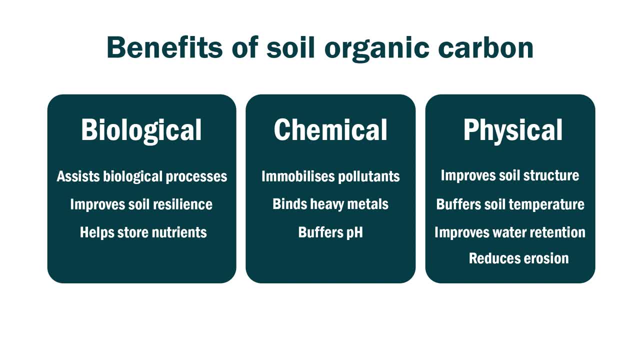 for the most part, it's the soil organic matter. So we use an estimation or an approximation of our soil organic matter based on those organic carbon measurements, And in doing so it gives us, finally, soil organic carbon becomes important because it's something we hear a lot about in 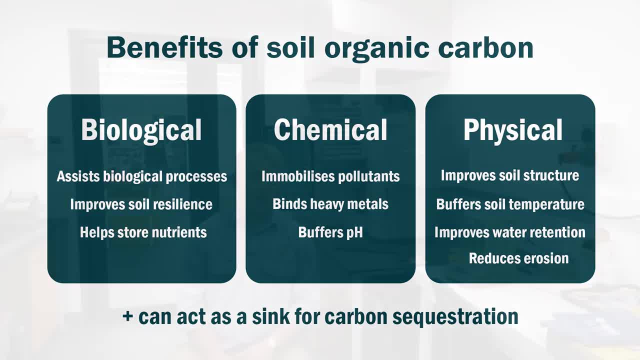 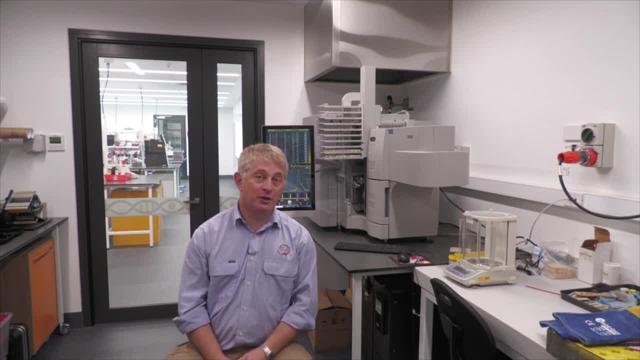 relation to our fight or struggle against climate change. Our ability to put more carbon into our soils is often something we're encouraged to do, And this is why we might want to look at our soil organic carbon. But in our soils that soil organic carbon can exist in two other forms. 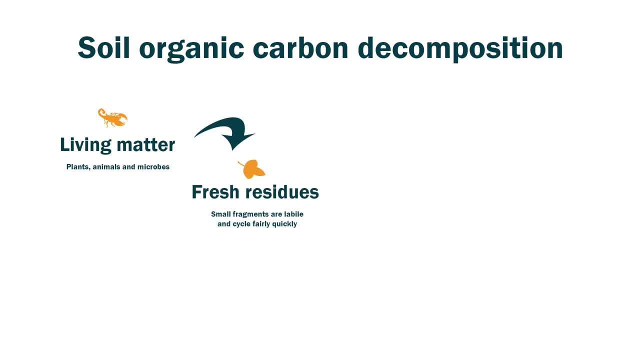 the labile form, which is what's feeding that biology and driving those nutrient cycles, and a recalcitrant form which is nearer to the inorganic often, but is more like humic substances, or what we call minerally occluded carbon. And that's the type.